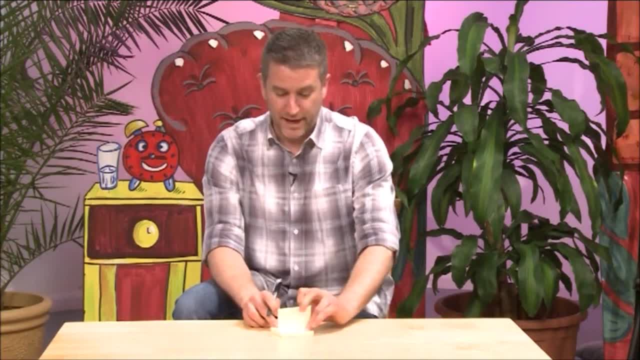 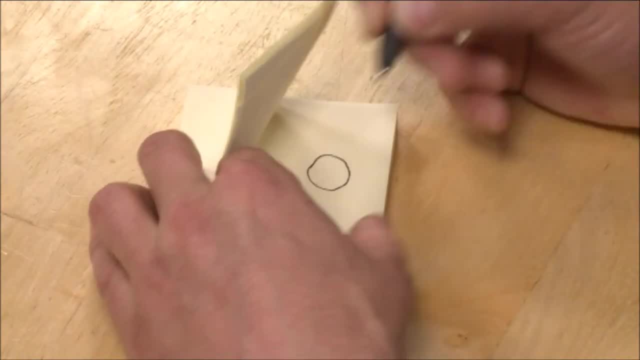 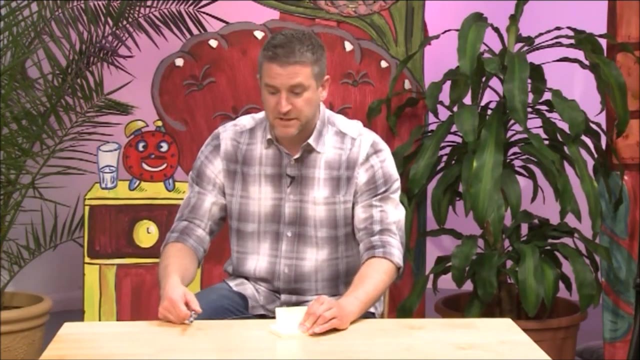 It opens up again into a full-shaped ball and starts to boing back up in the air. So now you can repeat that process with the ball going up again, and up again. Now you might be thinking: well, what on earth is he doing on all these different bits of paper? 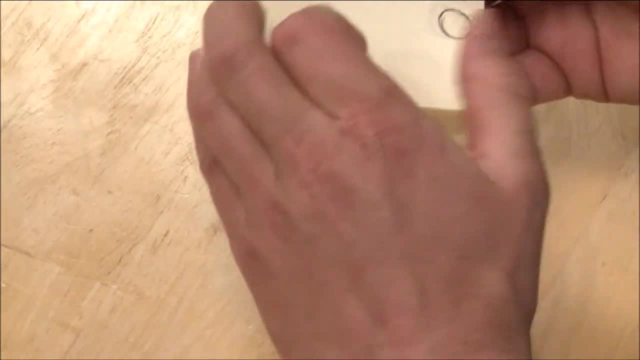 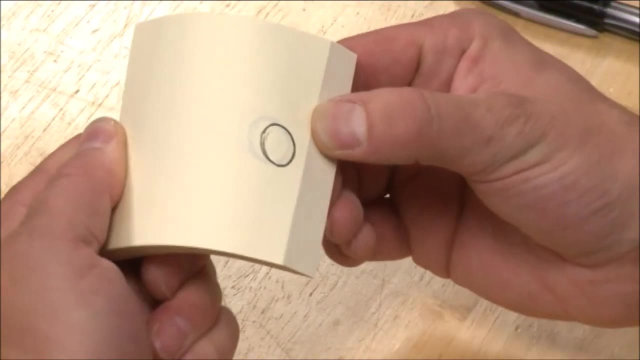 Well, let me show you. When you look at them in quick succession, one after another, if you flick through them, something fantastic happens. Watch this, Watch Boing. Did you see it move? It went up and down and bounced. 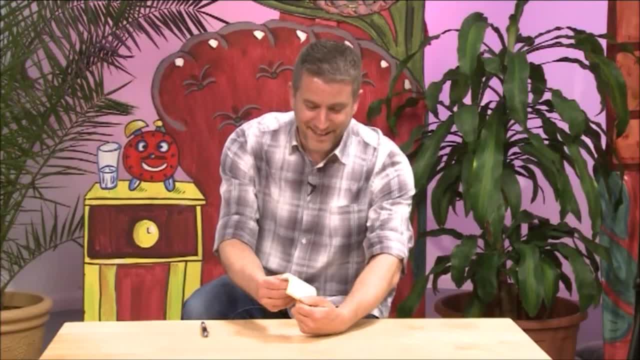 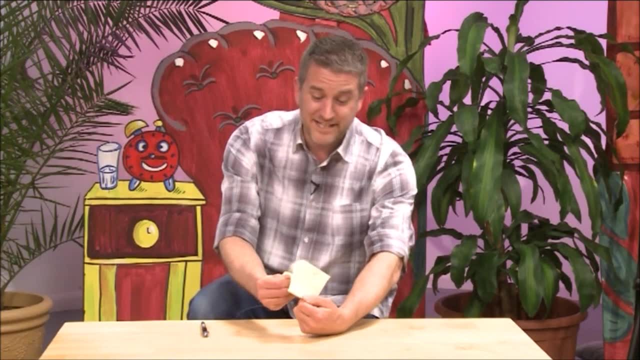 Boing. Hey, have a go at that at home. See if you can make your ball bounce on a flicker book. Isn't that fun? And that's the basics of how we make cartoons appear to move on the television. How's yours getting along, monkey? 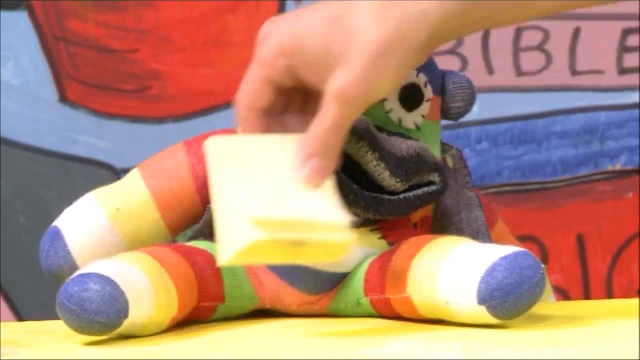 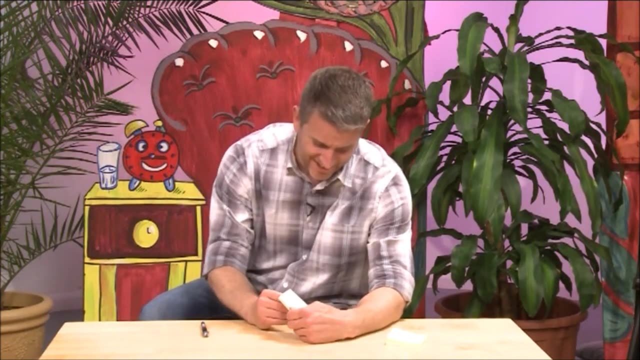 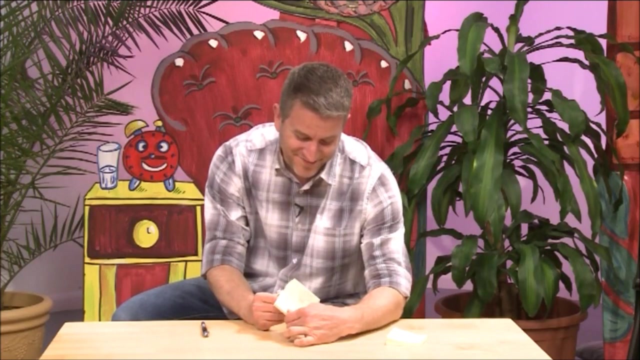 Can I have a look? There you go. What have we got here then? Hey, this doesn't look like a ball, It's got a face on it. Ah, Oh, my goodness me. What have you done, monkey? Look at that. 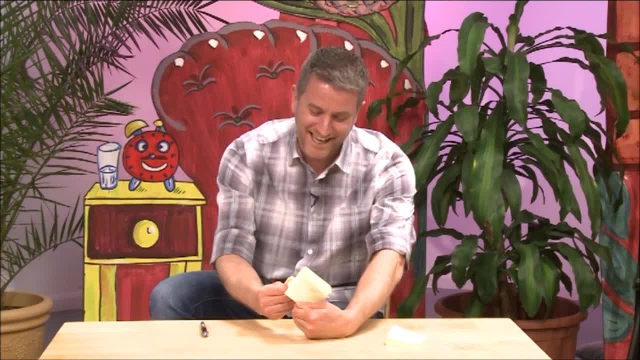 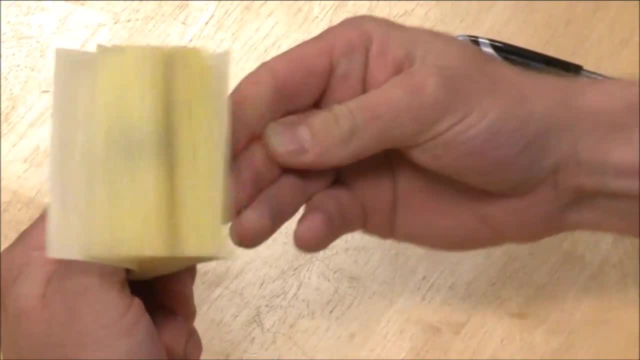 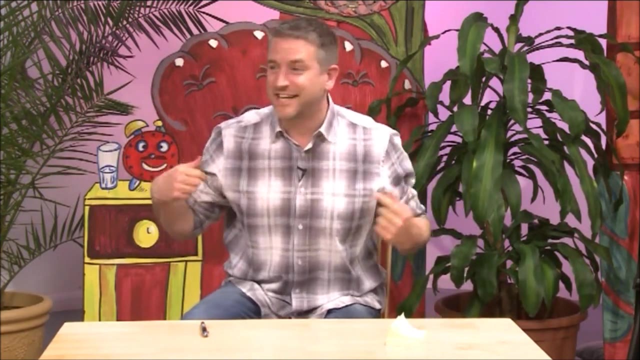 Oh no, you've done it again. How rude, Oh dear. Well, that's it. That's all we've got time for boys and girls. I hope you have loads of fun making your animations at home. That's it from me, Jovis Bon-Hovis, and these guys, the Creation Crew. 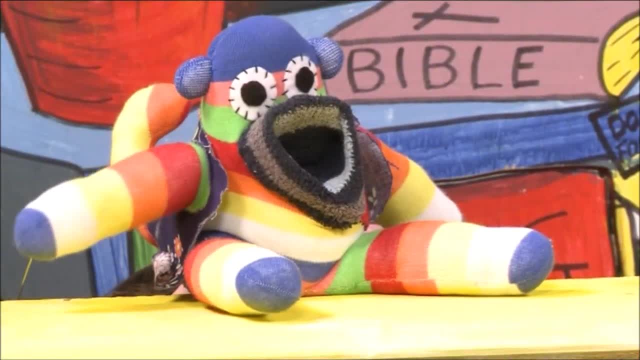 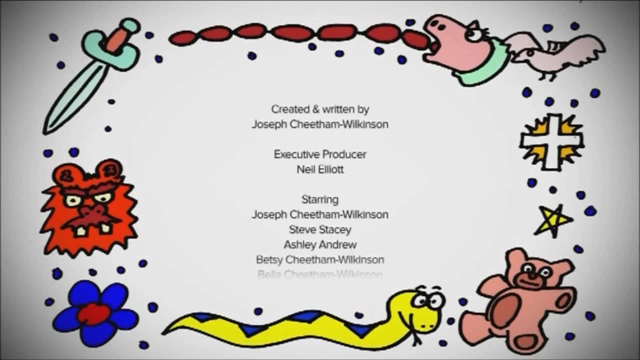 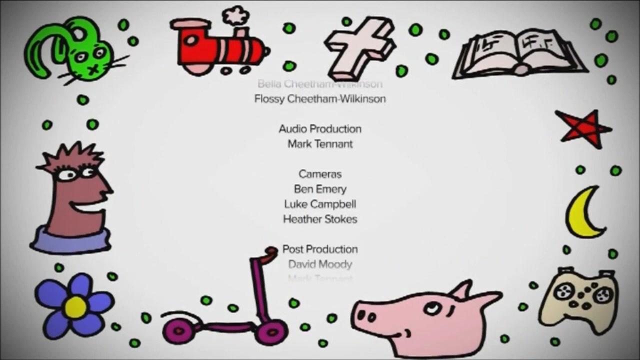 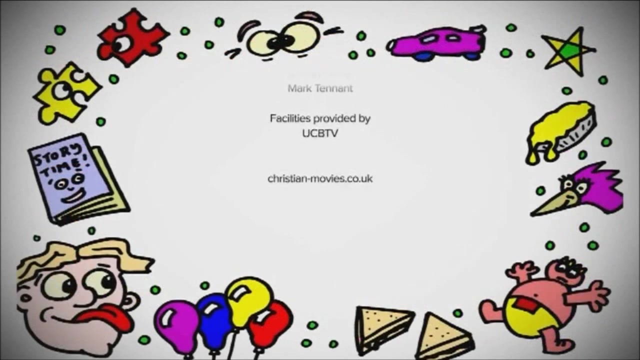 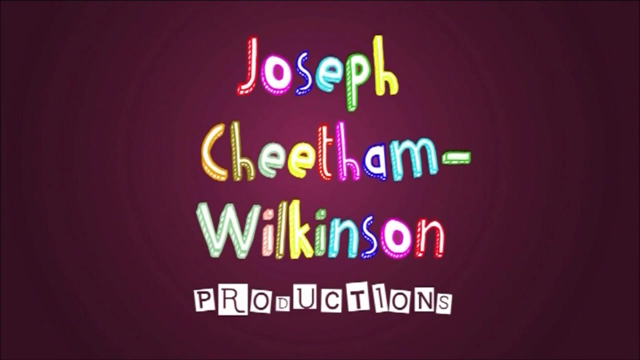 Bye, See you next time, Bye, Bye.